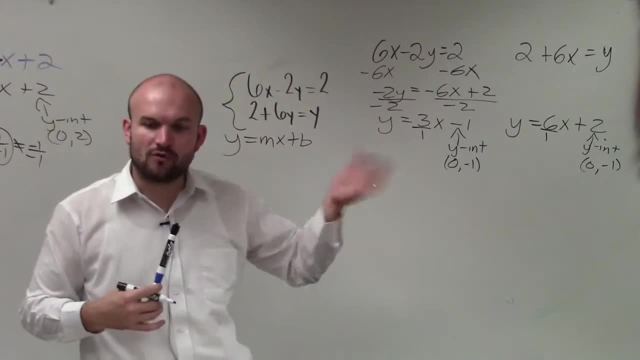 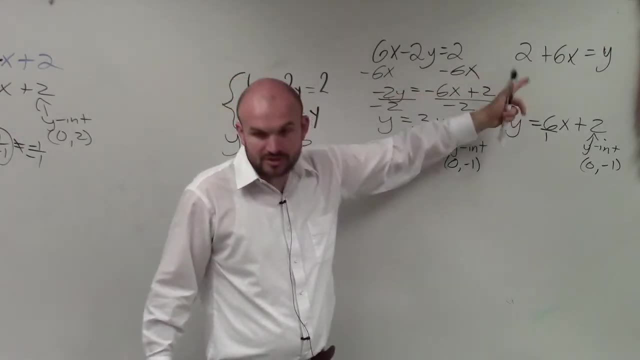 So if your slope is negative, if it's not already a fraction, put it over 1, so it is a fraction Again. change in y-coordinates over a change in x-coordinates. Change in y-coordinates over a change in x-coordinates. 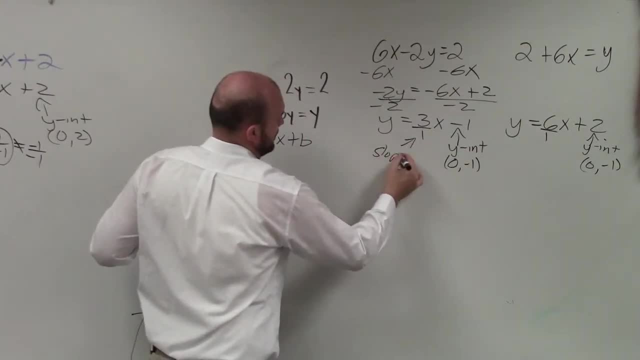 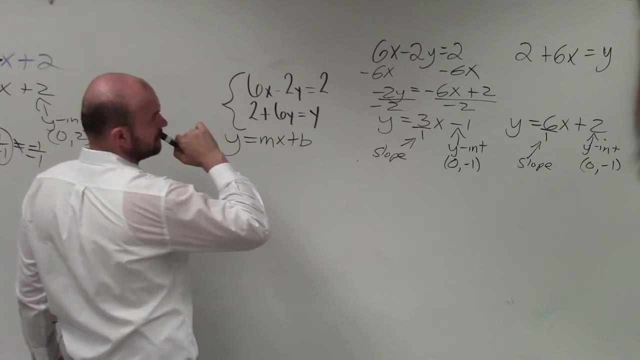 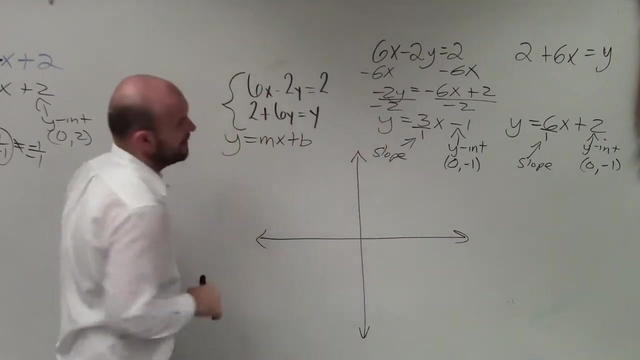 So now we know that information, Let's go ahead and graph them, Okay. So here, the first one I do is: I go to my. let's graph this one first. They both have this. what am I doing? That's 2.. 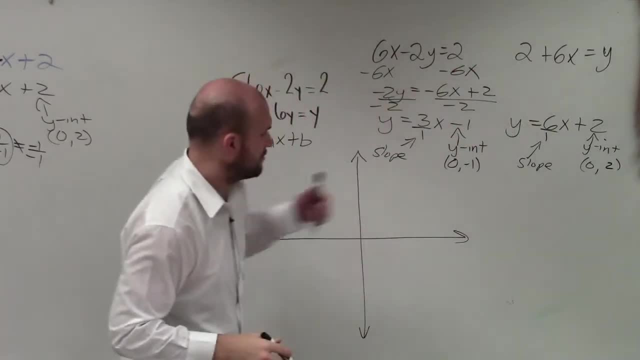 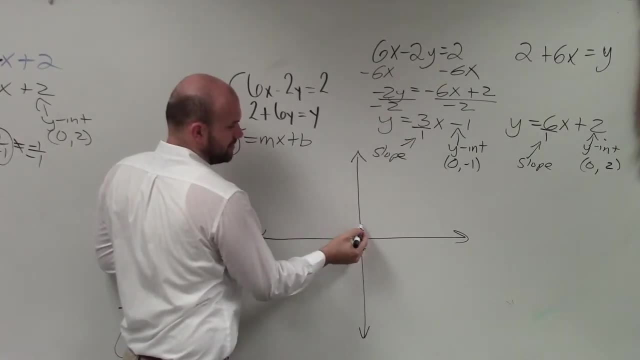 Geez, what the heck am I doing? All right, so this one has a y-intercept of negative 1. And then my slope is: change in y-coordinates is positive 3. So I go up 3.. 1,, 2,, 3.. 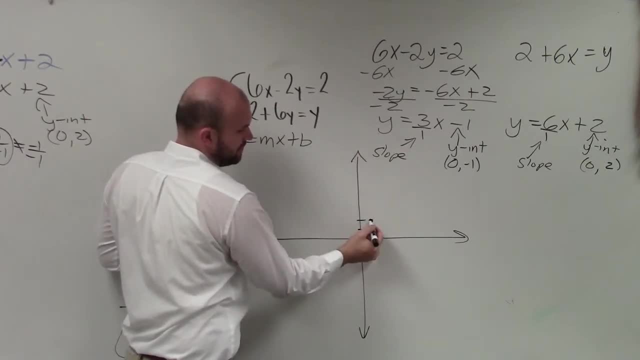 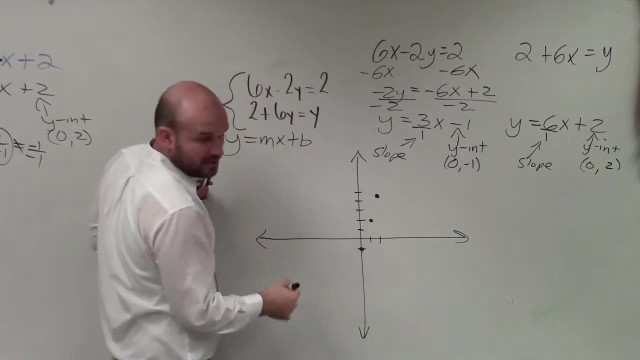 Change in x-coordinates is positive: 1. So I go over 1. So up, 3, over 1. I can just continue doing that. 1,, 2,, 3, over, 2.. Do you guys follow me? 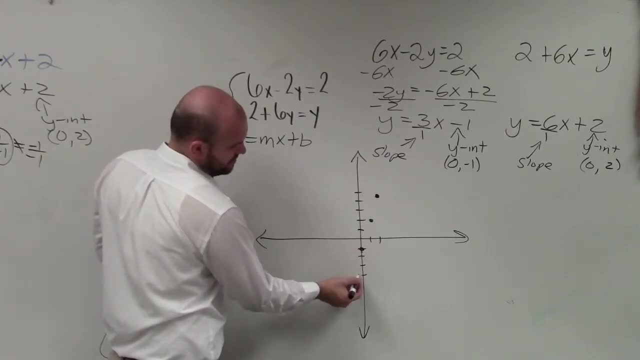 You could also go in the negative direction. You also go down 3.. 1,, 2,, 3, to the left one. You guys notice they all lie in the same line. Now let's go ahead and graph the next one. 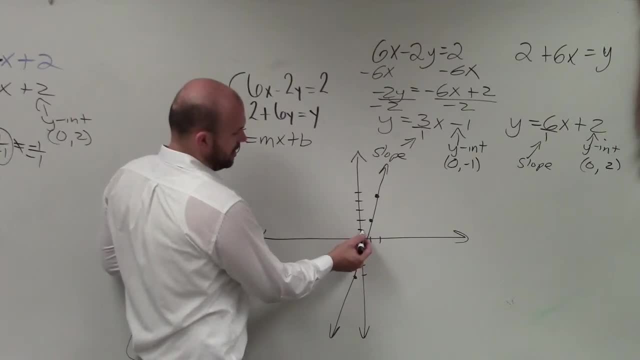 which has a y-coordinate of 2.. So up, 2.. And then this slope is change in: y is up 6. 1,, 2,, 3,, 4,, 5,, 6, over 1.. Then I go down: 6 over 1.. 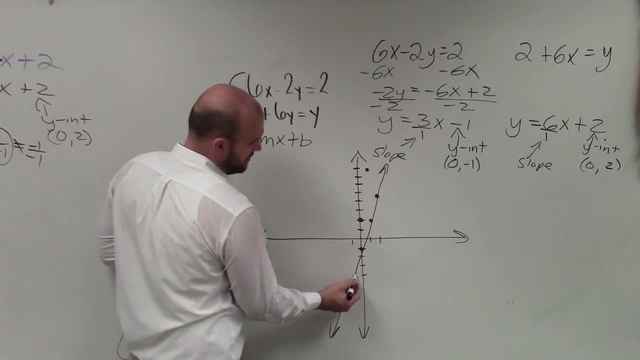 1,, 2,, 3,, 4,, 5, 6.. 1,, 2,, 3,, 4,, 5, 6, to the left one. So what I want you guys to notice is that these two lines intersect. 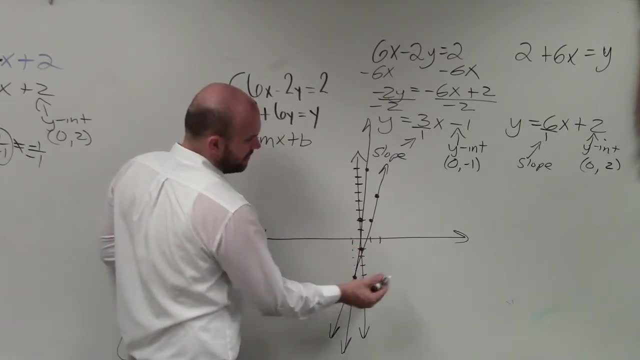 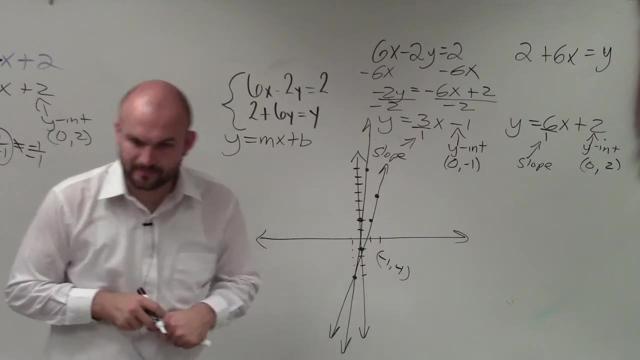 at the coordinate point: negative: 1, 1,, 2,, 3, 4.. Do you guys agree that that is their intersection? So that is your solution. Now I'm not going to go over.